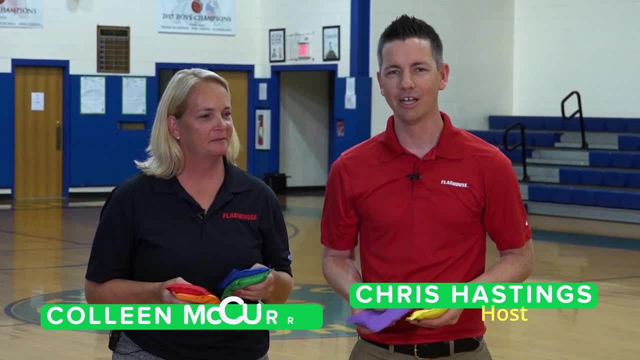 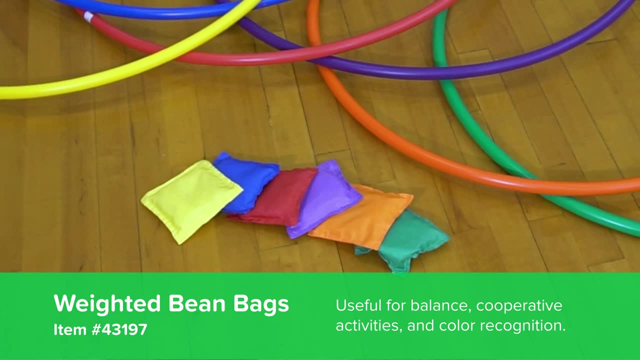 Hey everyone, it's Chris from Flag House, and this week I'm here with Coach Colleen McCurry to look at some instant activities that you can use with bean bags. Bean bags, I don't know about you. they're a staple item in our phys ed closet. We can. 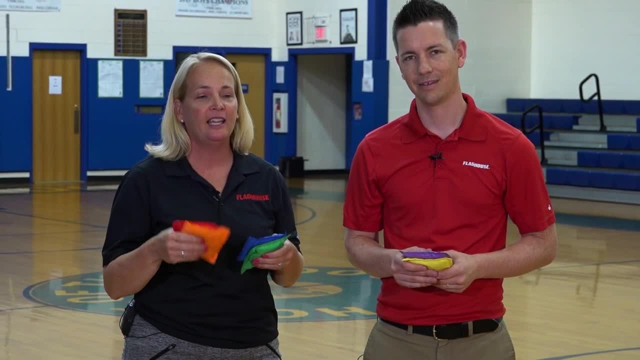 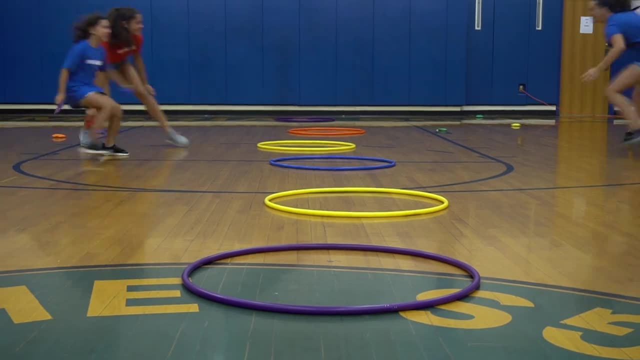 roll them out, use them for all different activities. It's a great way to get the kids in moving, doing physical activity, getting them warmed up and started for the day. as you're getting ready to do instruction, Try them out and throw them into your new instant. 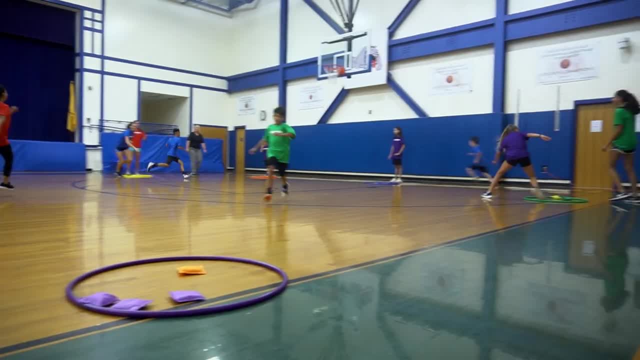 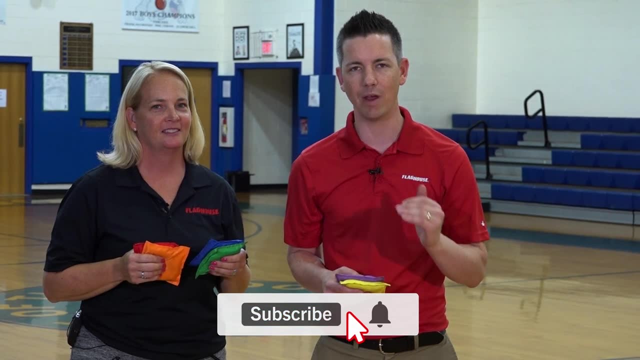 activities. So we've got these great instant activities coming up next. And hey, if you like videos like this, if you like activities like this, then you need to subscribe to the Flag House Activity Channel. We have brand new episodes with great ideas every single Wednesday Coming. 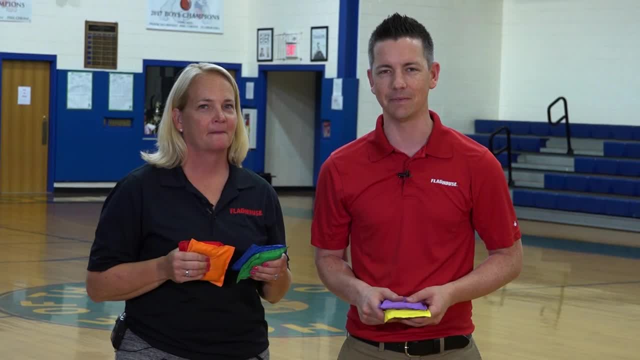 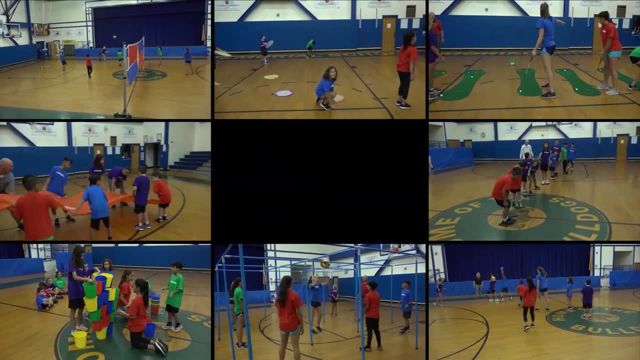 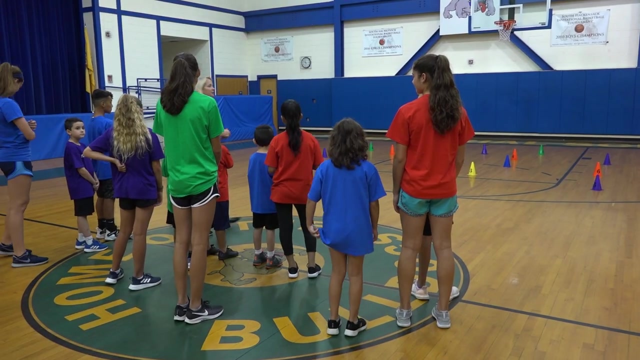 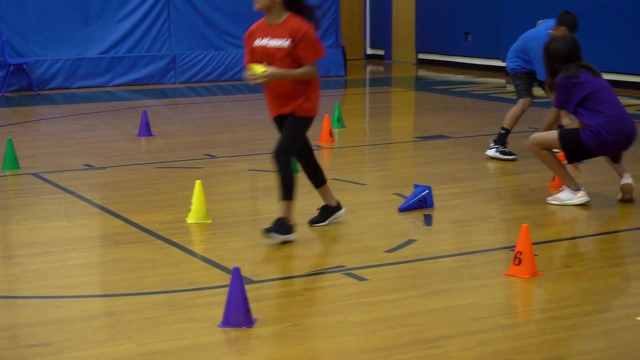 up. next it's instant activities using bean bags on the Flag House Activity Channel. So each group is going to be assigned a color. This is a warm up game As well as a memory game, right, Because you're going to jog out and you're going to turn. 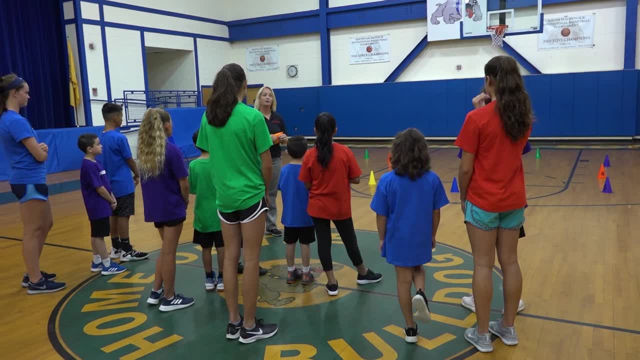 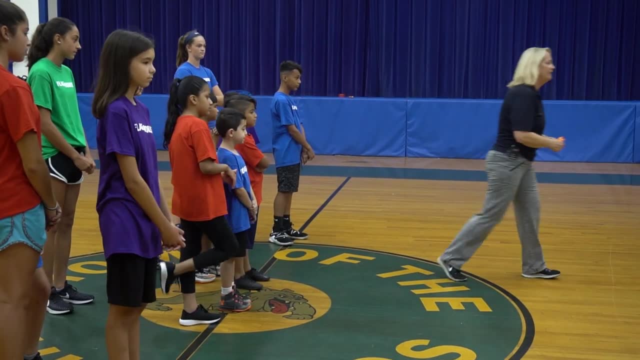 a cone over And if it has the color that your team has been assigned, then you're going to take the bean bag with you and run back and put it behind the line and tag off to the next person on your team. They're going to run out and they're going to flip over. 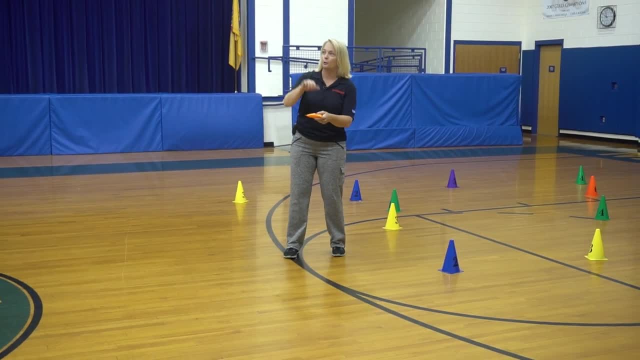 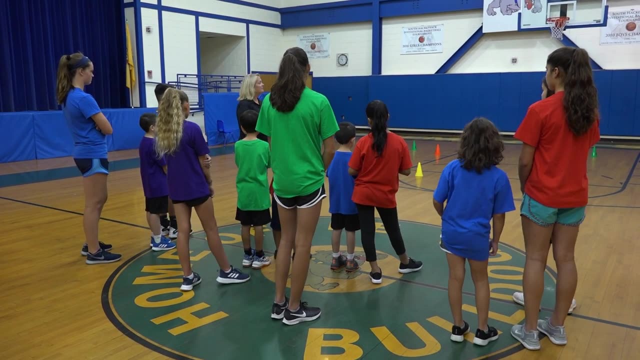 a cone. If it's not your bean bag color, you need to close the cone back up and cover the bean bag and run back and you go back and tag off to the next person on your team. So if it does have a bean bag underneath it that matches the color you've been assigned, then 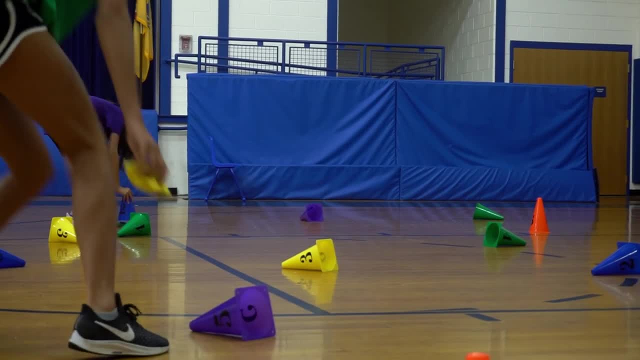 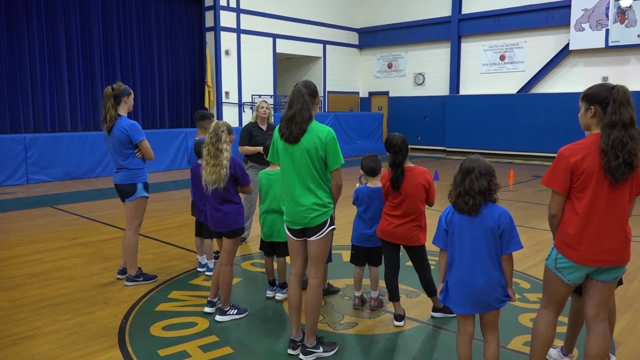 you're going to turn the cone on its side. Okay, So just to indicate that there's no longer a bean bag underneath there, there are four bean bags that are your team color. You need to get all four, And once you have all four, you're going to bring it over the 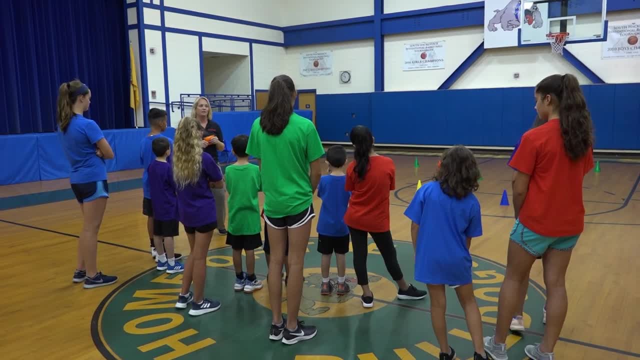 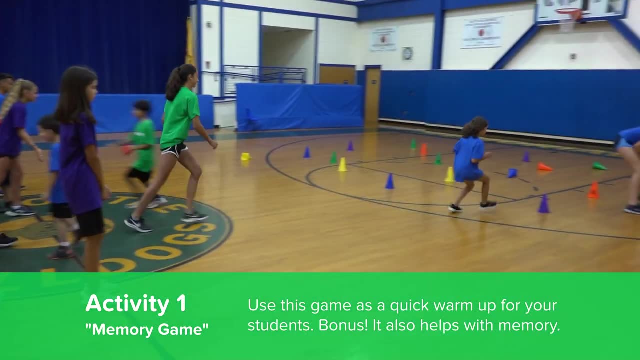 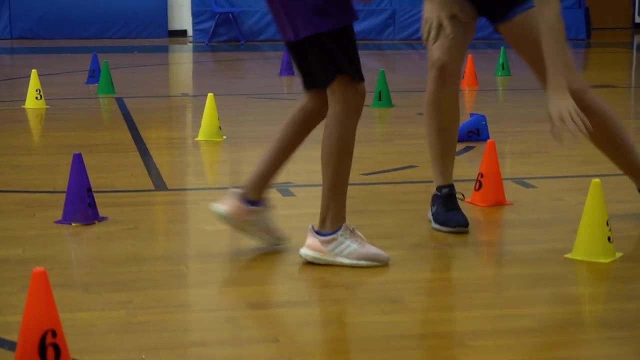 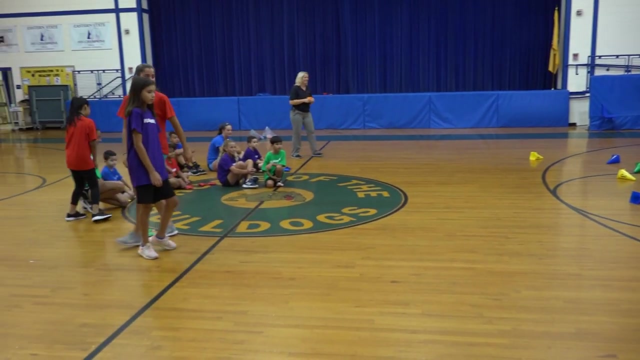 black line and everybody's going to sit down to indicate that your team has finished the challenge. Turn it on its side, Go back, turn it on its side. Somebody said, yeah, left it, left it up, All right, Great job. So this is a bean bag. 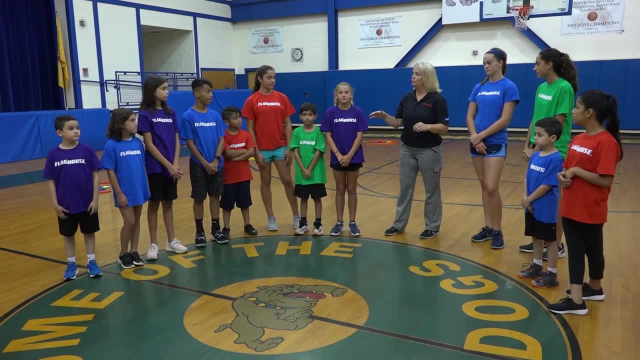 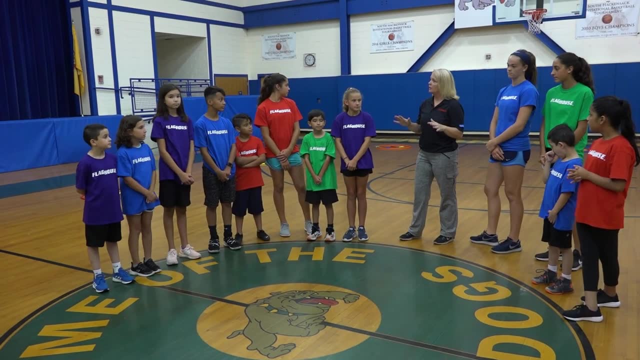 partner challenge and each group is going to be assigned a hula hoop and you're going to start off there and you're going to notice that there are different colored bean bags in your hoop and your color that matches your hoop is somewhere else. So what's going to? 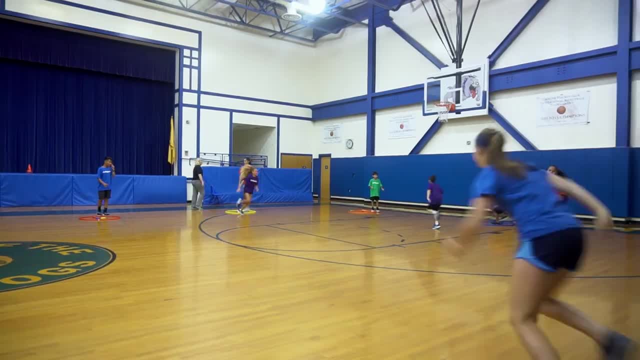 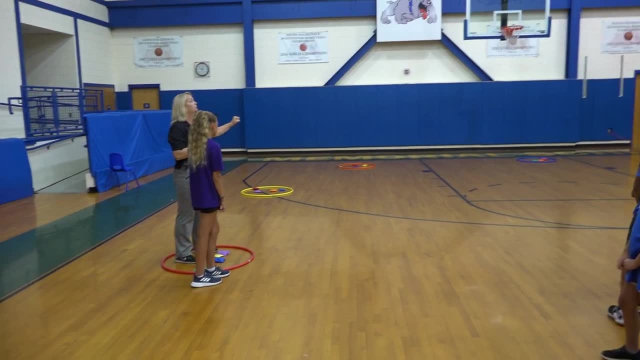 happen is you're going to have a partner tag off. right, We're here. She starts off, She needs to go find one of our red bean bags and she's going to run off. and she's going to go take a bean bag from another hula hoop. come back and drop it off, And right I'm. 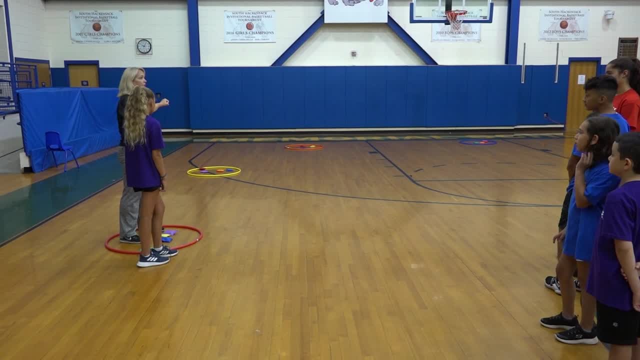 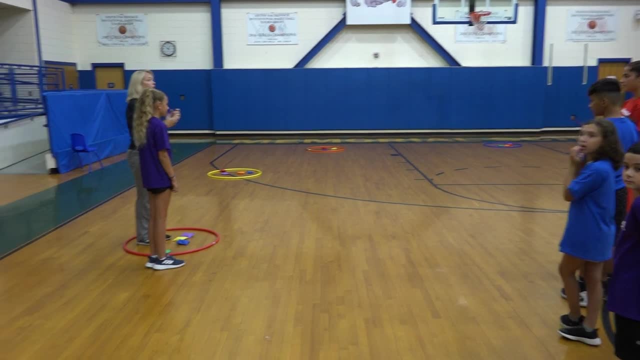 going to go She as soon as she comes back, I'm going to leave and try to go get another red and we're going to try to be the first team that has only red right Represented in our hoop to get our four. And, of course, if you're on the yellow team or the orange, 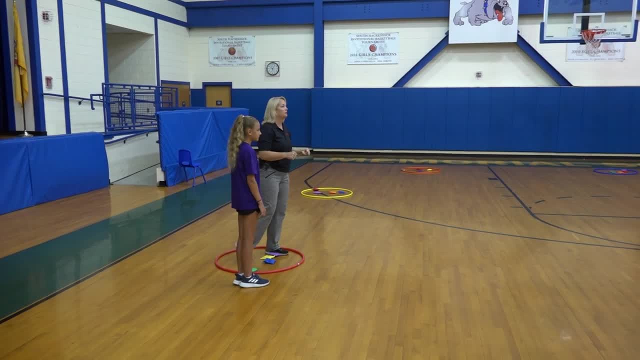 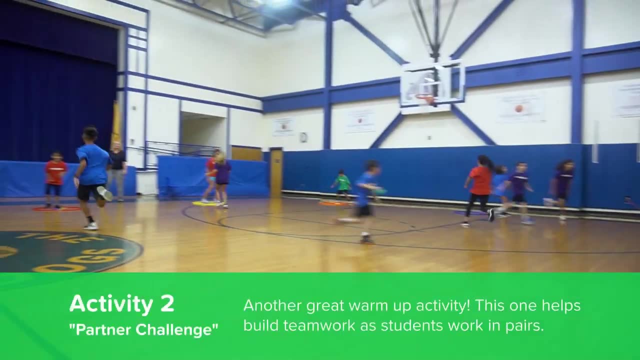 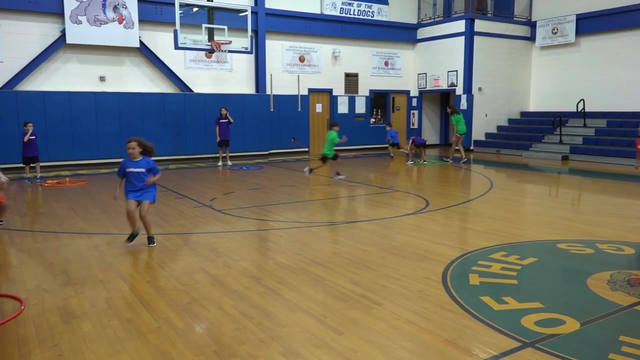 team. you're trying to get your bean bags and get them back in Back into your hoop So you have all four of your own color that match your hoop bumpers up. Make sure you're always looking forward, Make sure you're looking another way that you can do this game And it's okay If you. 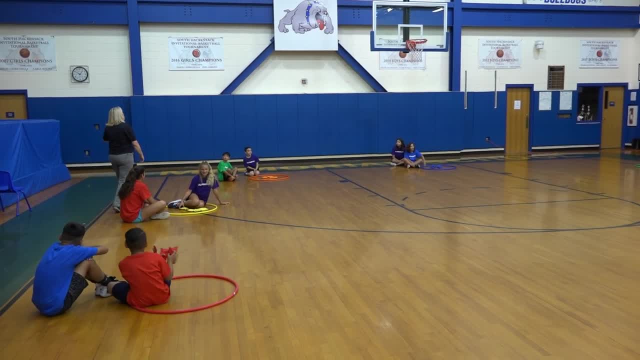 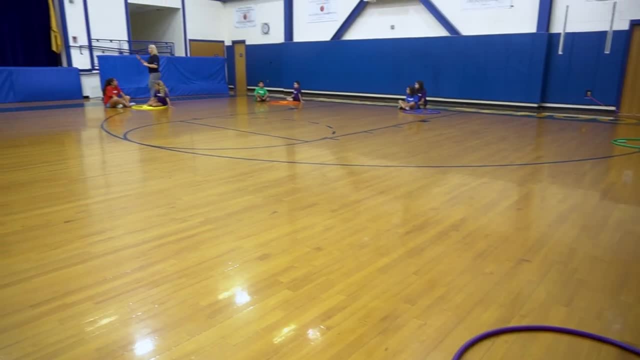 have all the same color. the goal will be for your hoop to be the first one that is empty. So you're going to leave and go drop a bean bag off in someone else's hoop And run back, and then you're going to take the next one and try to drop it off somewhere. 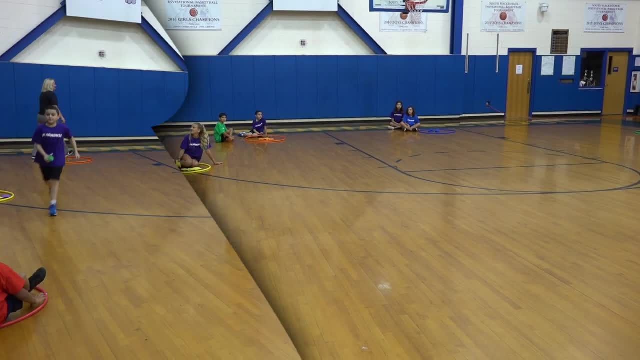 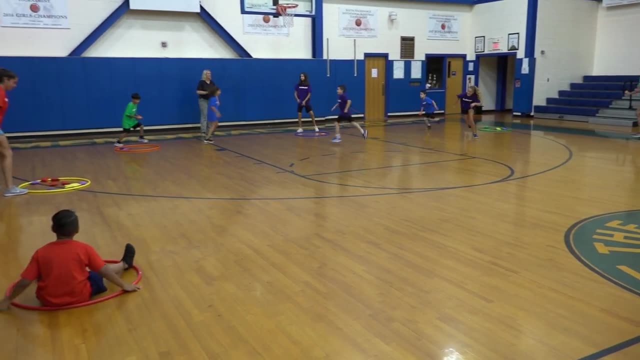 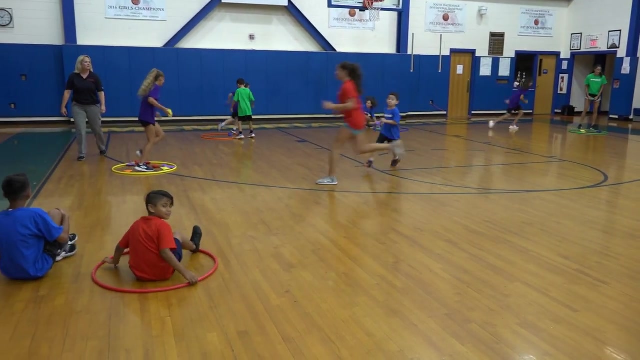 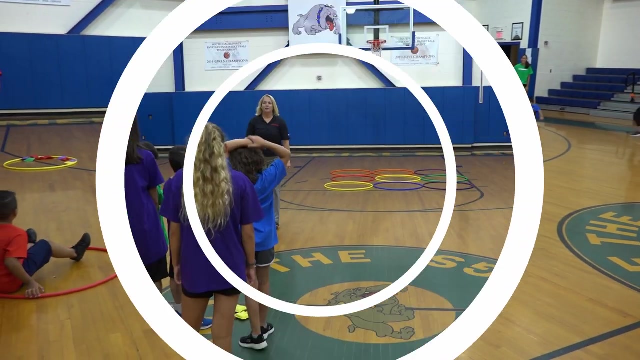 And you want to be the team that ends up with your hoop empty. There you go. Charlie's hoops looks awfully full. Oh, all right, And have a seat. We're going to start off. so say, for example, Michael is the first one in his line. 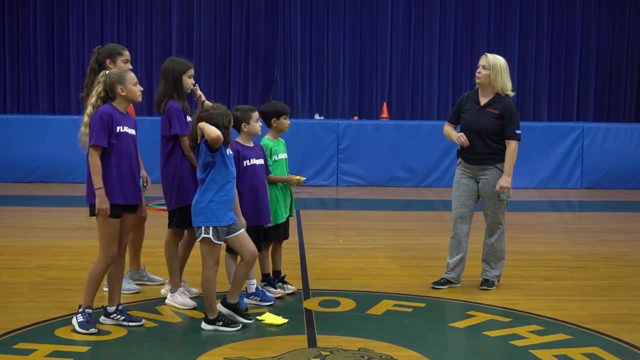 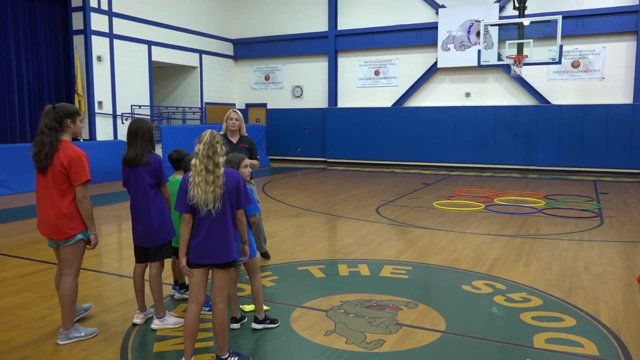 He's going to take one beanbag, He's going to run out to the tic-tac-toe board and he's going to drop his beanbag into one of the hoops And then he's going to run back and tag off to the next person on his team. 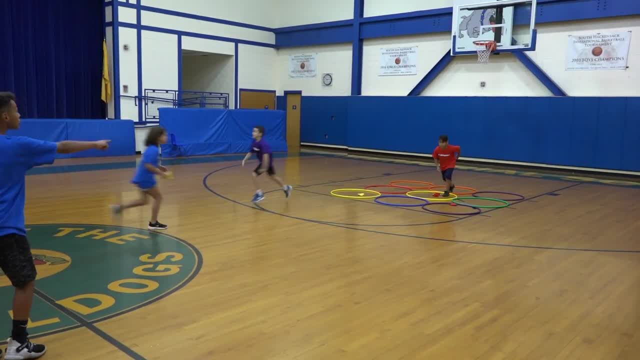 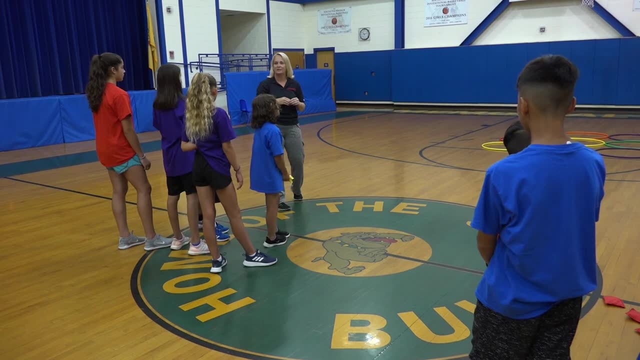 And then the next person will pick up a beanbag and run out. So if there are no beanbags for you to carry down when you get there, you can pick your beanbag up and put it in a new location to try to create tic-tac-toe for your team.